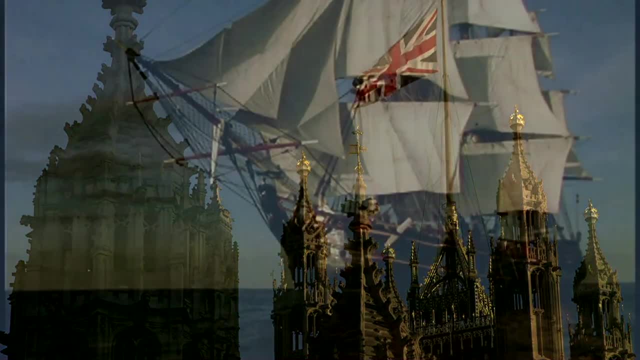 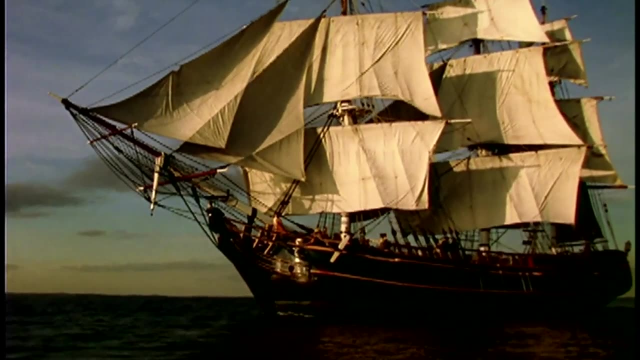 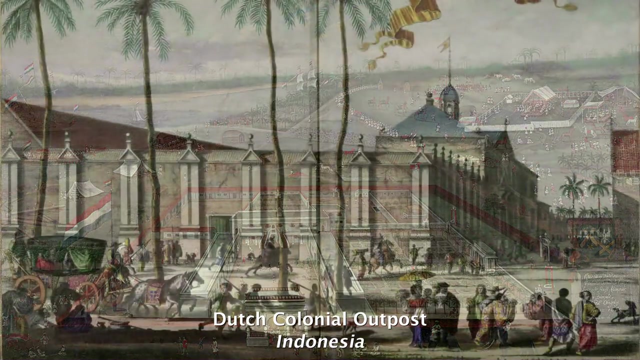 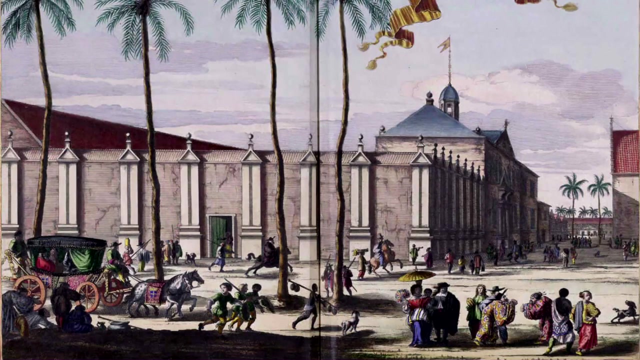 This is due to the fact that, hundreds of years ago, certain powerful European nations carried out intensive programs of world exploration that led to their colonization of far-distant lands. Because of their colonies, many aspects of European culture, including legal systems, languages, religions, art, architecture and even ways of dress, were introduced to countries all around the world. 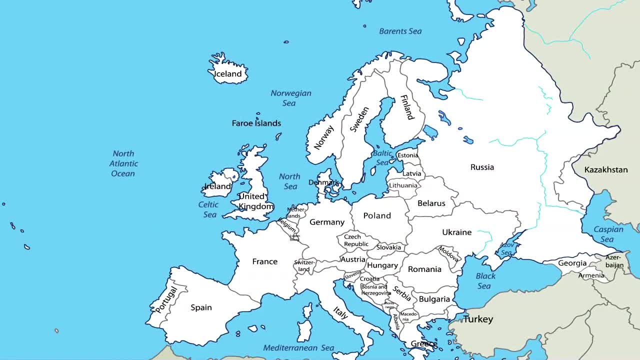 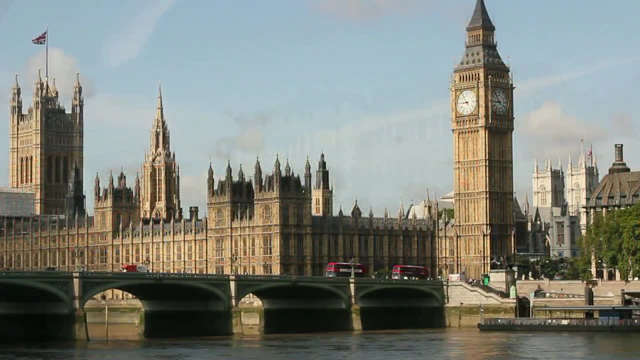 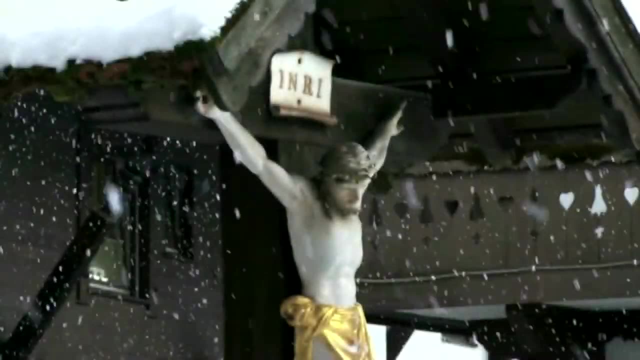 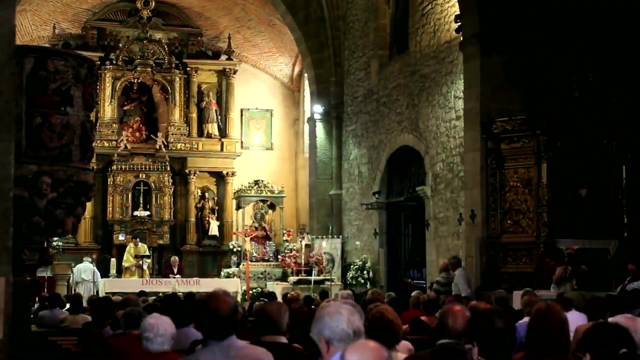 Today, the territory of the European continent is divided. It is divided up into 50 independent nations in which more than 100 native languages are spoken In Europe. almost all of its governments are democratic republics or constitutional monarchies. Christianity is by far the predominant faith in Europe and has profoundly influenced its thought and culture for well over a thousand years. 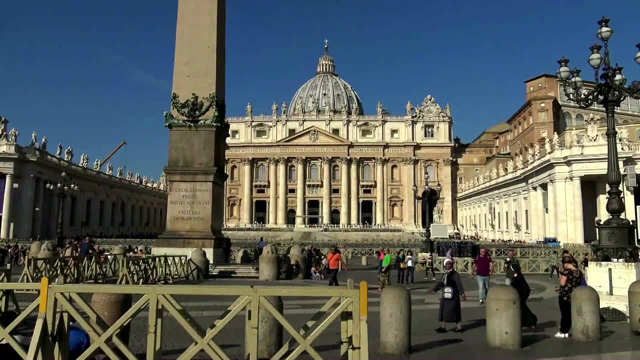 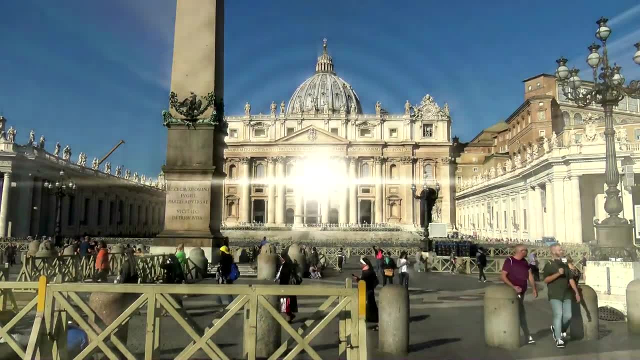 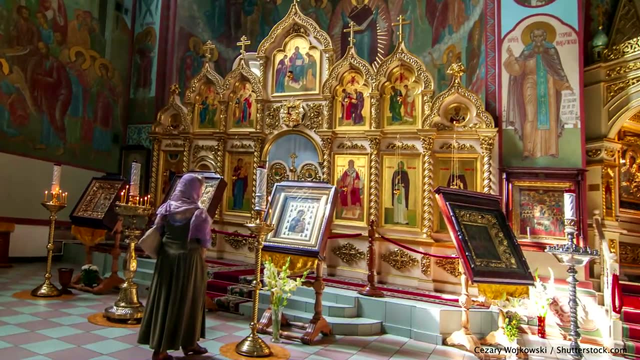 Most of the countries in the southwestern parts of Europe have deep roots in the Roman Catholic Church, The Roman Catholic Church which is headquartered in Rome in the Vatican City. While in northern Europe a large number of people are Protestants, In the more eastern parts of the continent many belong to the Eastern Orthodox Catholic Church. 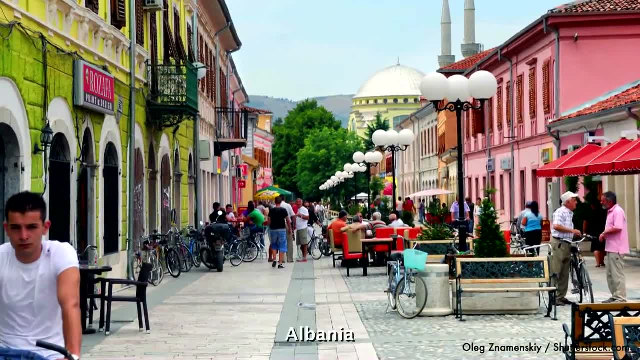 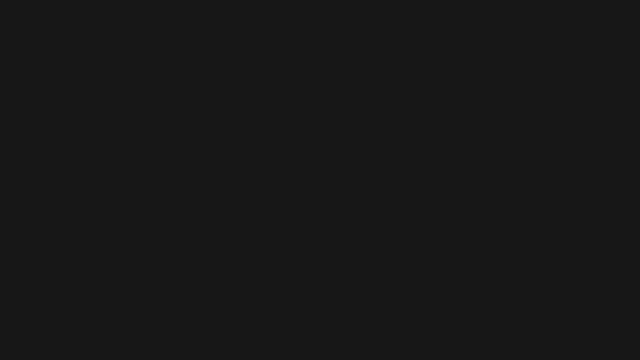 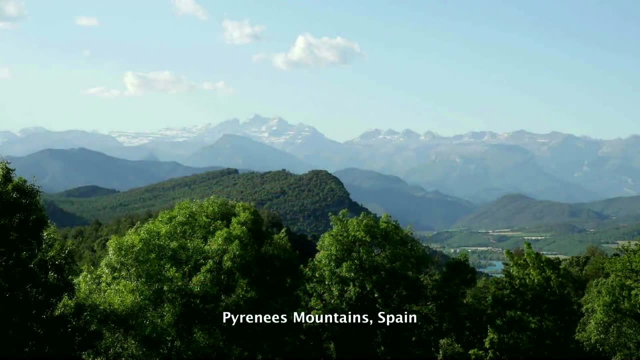 A few of Europe's Balkan peninsula nations, such as Albania, seen here, have Muslim-majority populations. Geographically, Europe's western and southern regions abound. Most of these regions are surrounded with mountainous and hilly terrain, and most of these lands are heavily forested. 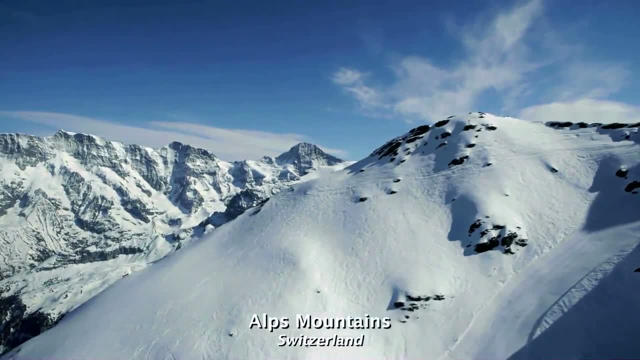 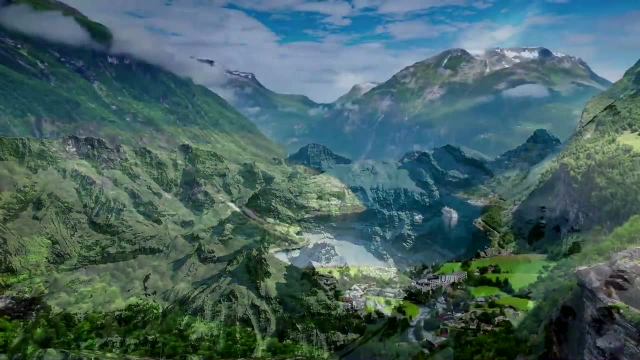 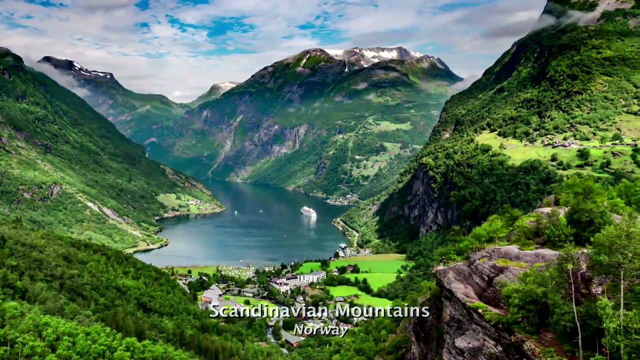 The Alps, which stretch across eight different countries, are the continent's most extensive and tallest range of mountains. With the exception of the lower elevation mountain ranges of Scandinavia, Poland and Slovakia, the majority of northern and eastern Europe consists of fairly flat plains, most of which are used for farming. 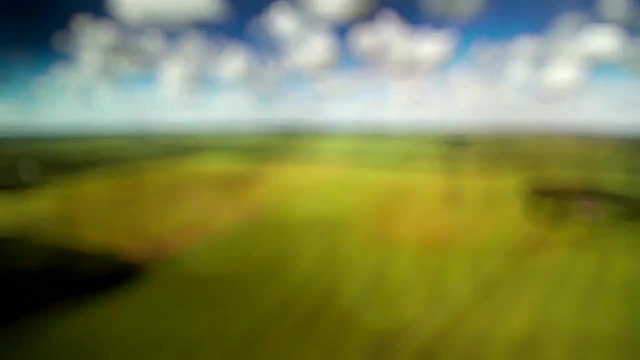 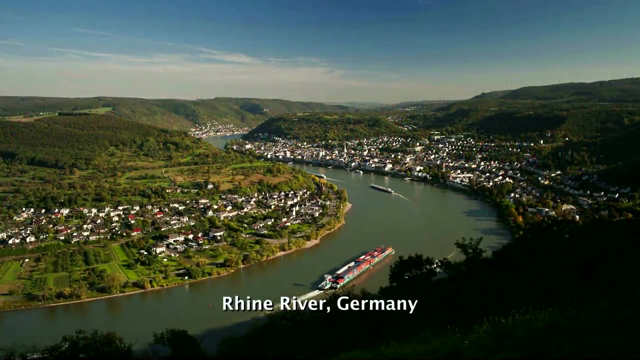 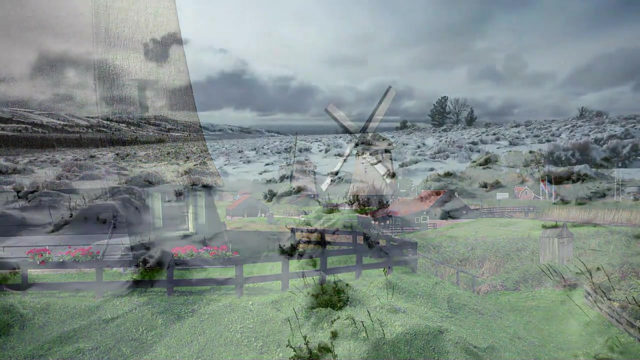 Climatically, Europe receives a fairly significant amount of precipitation, and that's why the continent has so many large navigable rivers and why it lacks any real deserts. A small percentage of Europe extends above the Arctic Circle, but most of its territory lies in the temperate zone. 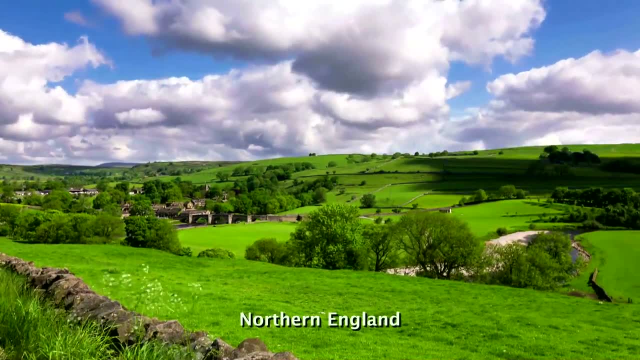 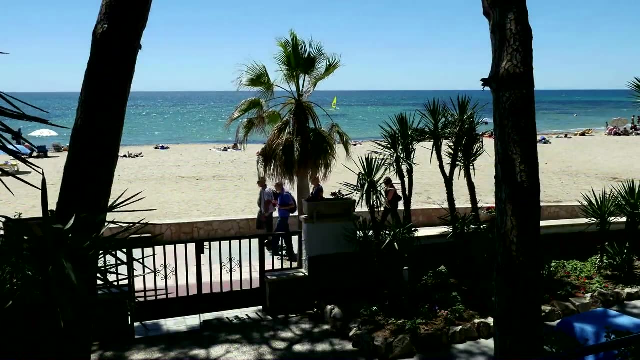 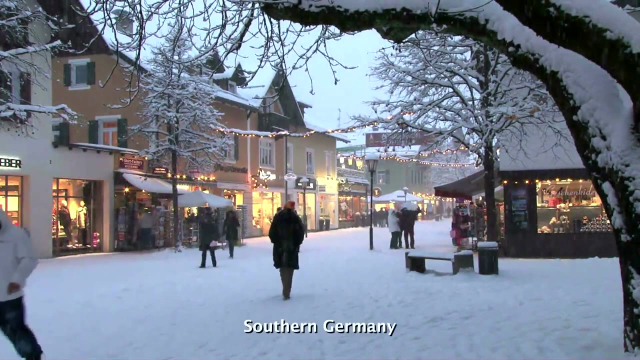 As a result, for the most part, the European climate is relatively mild. Nearer the Mediterranean Sea, the European climate is much warmer than in the north. However, further away from its coasts, in the continent's interior regions, more extreme temperature variations can occur.